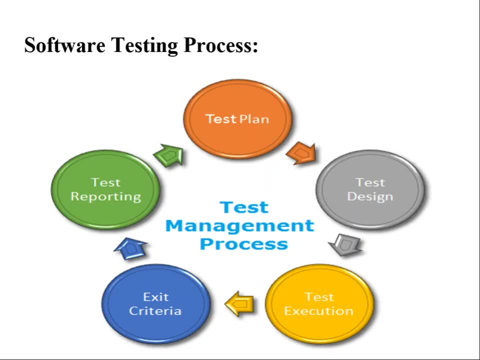 are there. all these informations is included in test plan document. by considering the test plan document as a basis, test design is going to be prepared. depending on test design document and considering it as a basis, test cases are going to be executed after performing the test cases. finally, exit criteria is going to be validated and then all the testing activities. 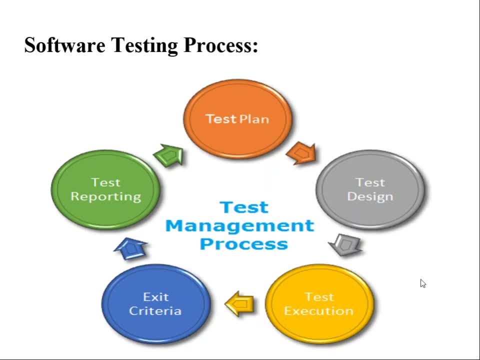 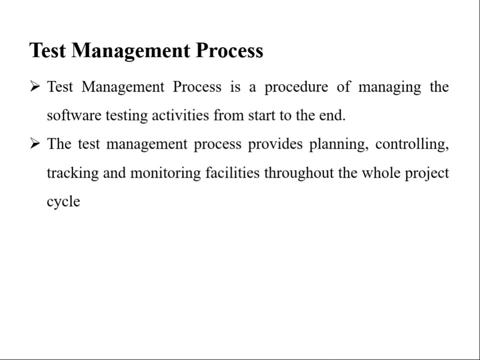 software testing process is going to be reported to the test engineer, test management team and to the end user by providing a one document which is called as a test summary report document. so these are the different phases of software testing operation. now test management process. test management process is a procedure of 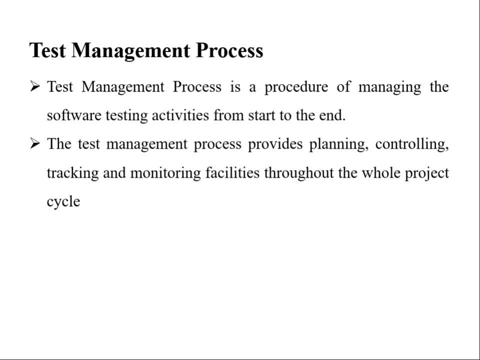 managing the software testing activities from start to the end. the test management process provides planning, controlling, tracking and monitoring facilities throughout the whole project cycle. the process involves several activities like test planning, designing and test execution. it gives us an initial plan and discipline to the software testing process test 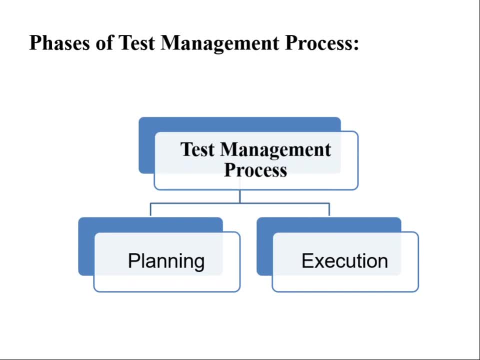 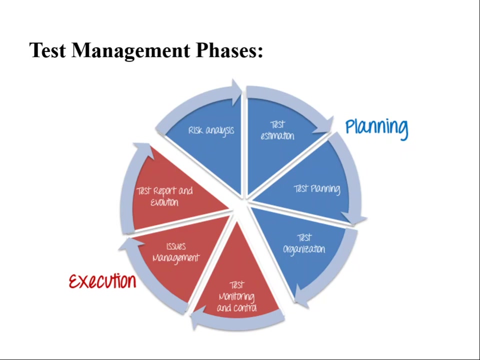 management is not just a single activity. it consists of series of activities. there are two main parts of the testing management process. first one is known as a planning and second one is known as a execution. under planning, it is divided into four different sections. first, you have to analyze the risk. then 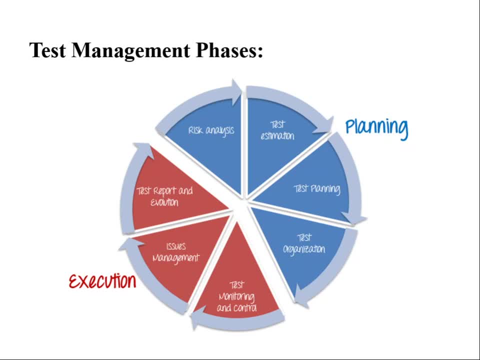 you have to estimate the testing operation, then prepare the test plan document and then organize the test testing operation. second part is known as a execution. second phase of test management is execution, where it will be divided into three main types. first one, test, monitoring and control. second, you have to manage. 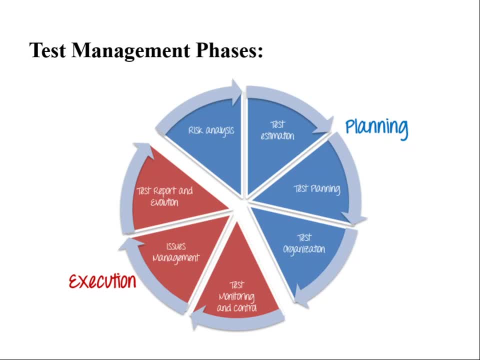 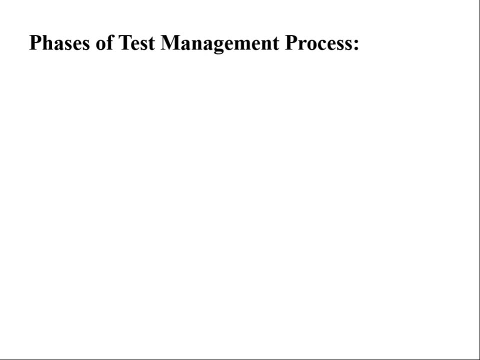 the issues involved in testing operation. and third, you have to report and evaluate the testing operation. now we will be discussing each of the phase of test management in brief. the first phase of test management process is planning under planning. the first point is risk analysis and you have to find out the solution on it. so what is risk? risk is is the potential loss. 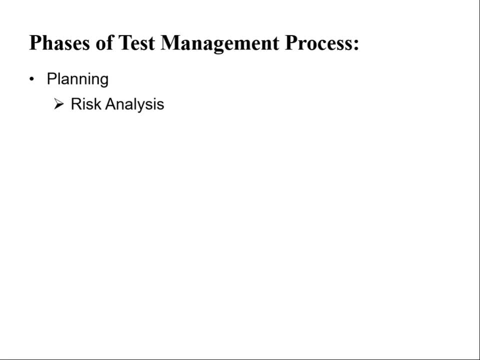 resulting from a given action or an activity. risk analysis is the first step which test manager should consider before starting any project, because all projects may contain risk. early risk detection and identification of its solution will help test manager to avoid the potential loss in future and also it saves the project cost also and time also. the next point: 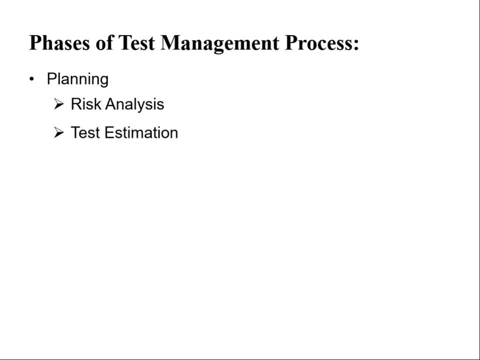 under planning is the test estimation. so an estimate is the forecast or prediction. it is an approximately determining how long a task would take to complete. it also estimates the efforts for the test, one of the major and important tasks of the test management. there are different benefits of test estimation. first, is it accurately? 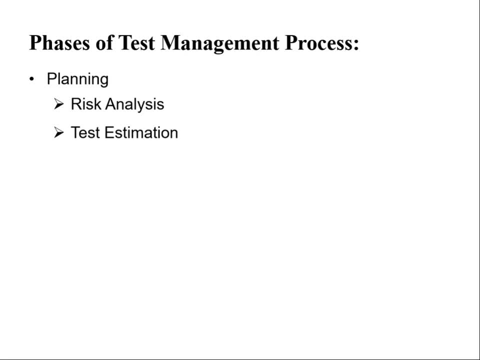 find out better planning, execution and monitoring of task under a test manager attentions. it also allow for more accurate scheduling and help realizing result more confidently. the third phase of planning is test planning. a test plan can be defined as a document which describe the scope, approach, resource and schedule of testing activities. 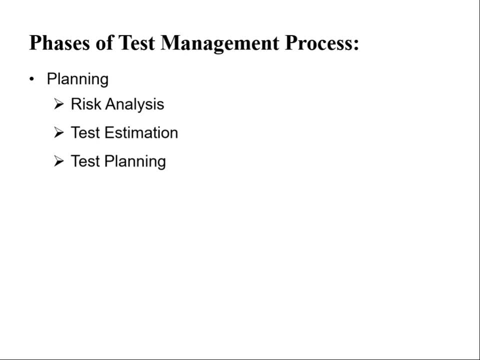 a project may fail without a complete test plan, so particularly it is important in large software system development. it includes test strategy, test objective, exit or suspension criteria, resource planning and also test deliverables. the next part of planning is test organization. so test organization in software testing is a procedure of defining roles in the testing process. 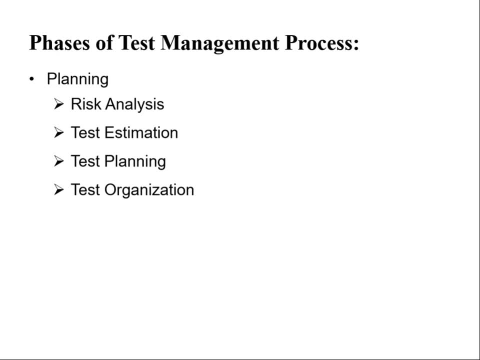 it also defines who is responsible for which activity in testing process. test functions, facilities and activities are also explained in the same process. now the second phase of test management process is execution under execution. our first point is test monitoring and control. so test monitoring and control is the process of overseeing all the metrics necessary to ensure that the project is. 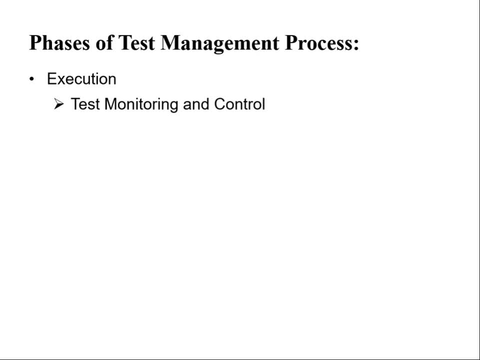 running well, on schedule and not out of budget. the next part of execution is issue management. in case of issue management, you are going to mention in the beginning of all topic what all projects may have potential risk. so when the risk is met, risk happens, it becomes an issue. 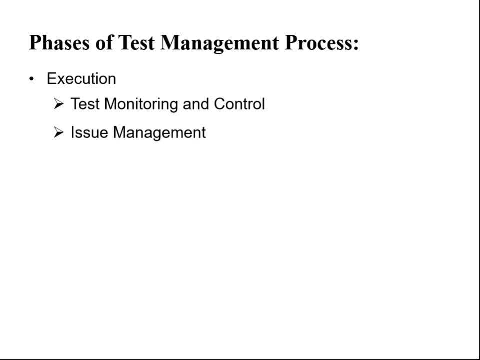 Risk is avoided while testing. you can check while missing the deadline. you can check whether exceed the project budget or also you can check with the loss of customer trust. Now the last phase of execution is test, report and evaluation, As all the activities of software testing is going to be completed. the last point is: